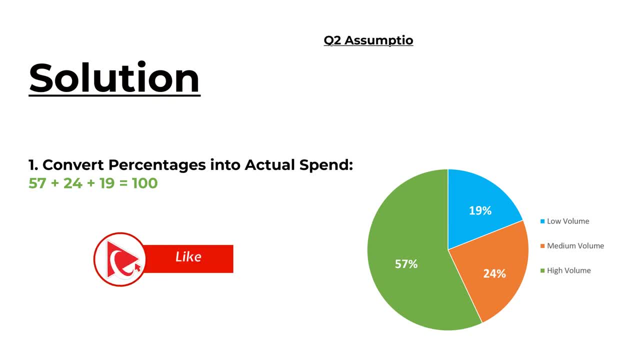 plus 24 plus 19 would be equal 100.. Now in the next step, we can calculate total planned spending in quarter 2. 57 for high-volume customers will remain the same, But we know that the medium-volume customers will spend half, And half of 24 is 12.. And then we know: 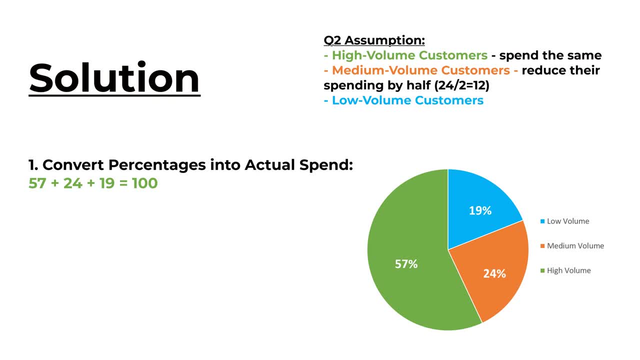 that the low-volume customers are planning to double their spending, which would be equal 19 multiplied by 2 as 38.. That's the last equation, Am I right? So the current equation of 25,000 plus 19 would be equal to 25,000 times 12.. And the 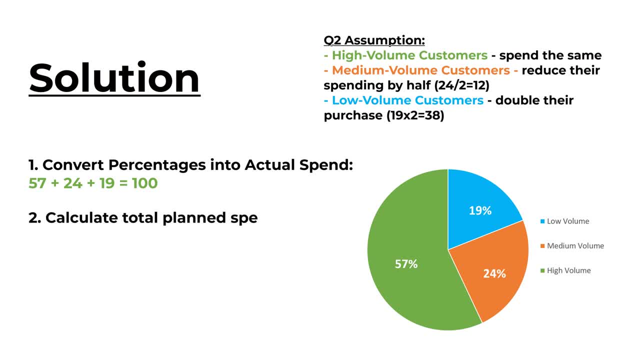 volume value of 50 will be equal to halfway over 5,000.. For a matter of fact, we need to, so the new equation will be 57 plus 12 plus 38, which would be equal 107.. To calculate Q2: 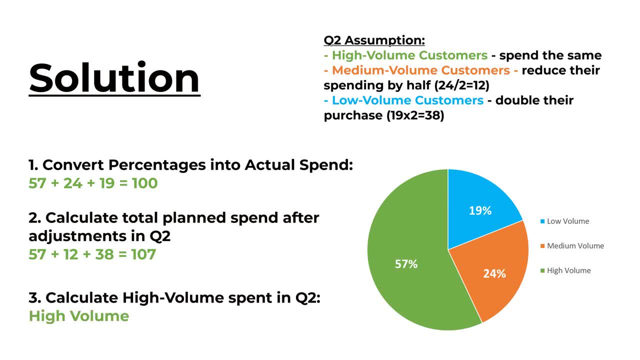 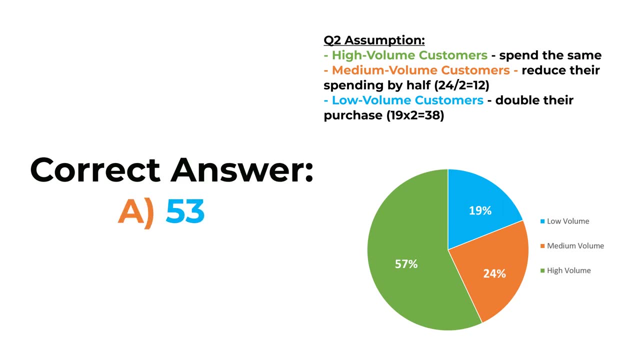 percentage spent for high-volume customers. we need to divide 57 by 107 and multiply it by 100%, so the new percentage value is 53.27%, which matches closest the choice A. So the correct answer here is choice A, 53%. Hopefully you've nailed this question and now know how to answer. 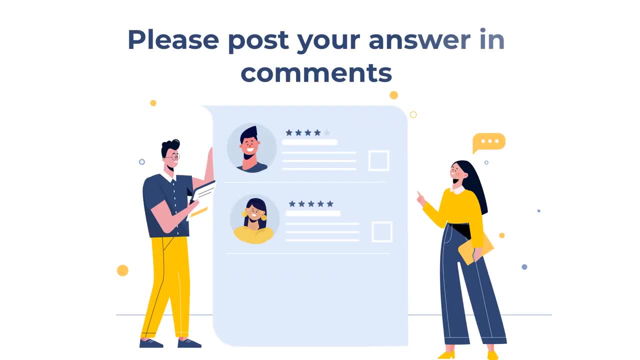 similar problems on the test. Do you have a faster way to solve it? Please make sure to post your solution in comments, And if you're looking for more questions to practice for the test, please make sure to check the description of this video for additional resources. 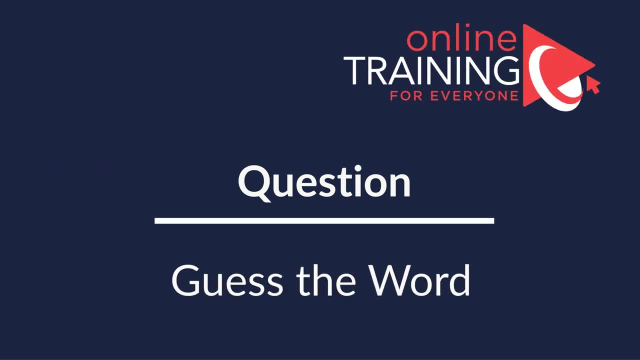 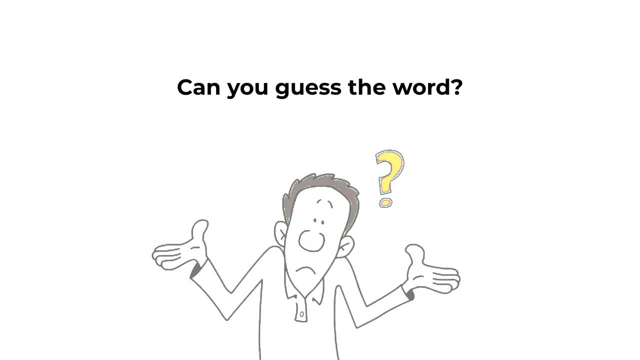 Here's the cool question that you frequently get on the test. You're presented with four different letters and you need to guess the word using all letters presented. The letters we have are W, O, B and L. Can you guess the word Give yourself? 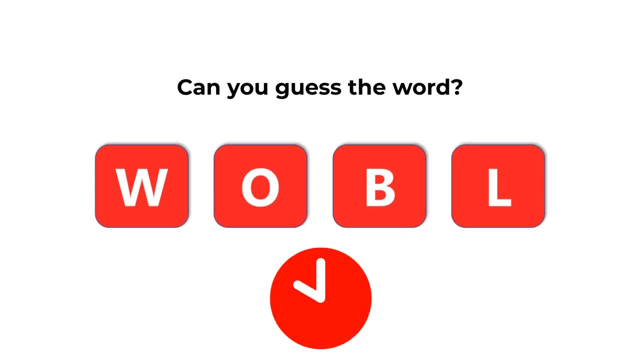 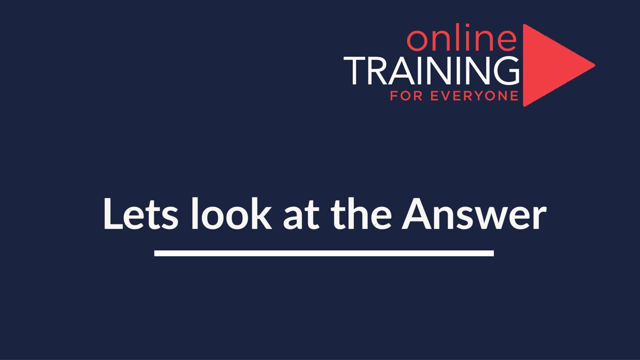 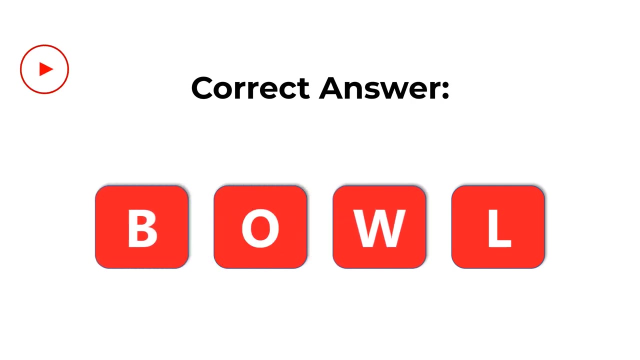 10 to 15 seconds to see if you can come up with the answer. Ready or not, let's go ahead and reveal the solution. The correct answer here is ball, which is spelled as B, O, W and L. Hopefully. 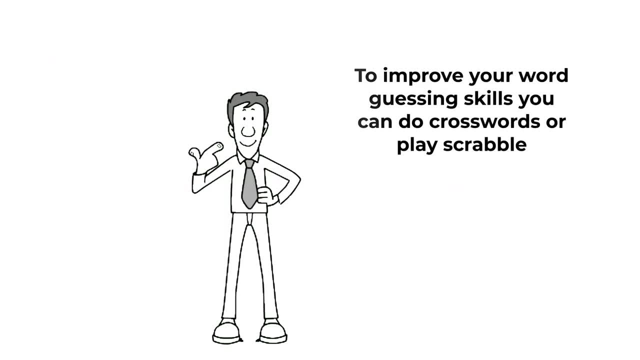 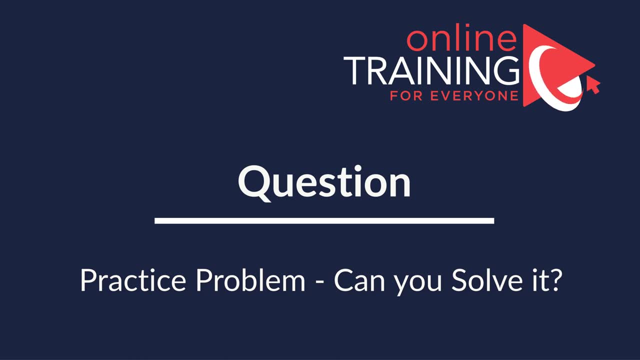 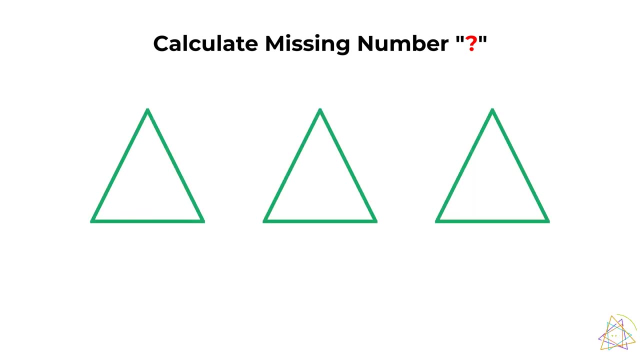 you've nailed it. Here's the question for you to practice. If you calculate the answer to this question, please make sure to post it in the comment section of this video. You need to calculate missing number and you're presented with three triangles. Each triangle has numbers in the 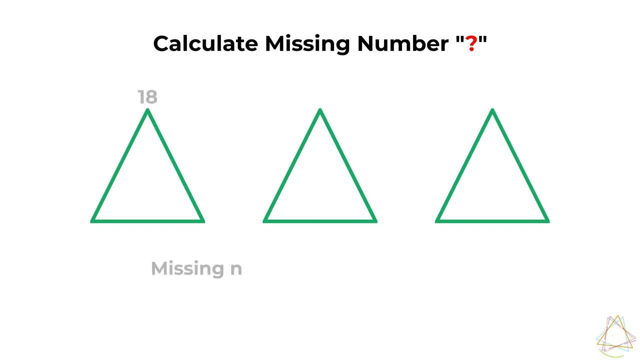 corners, as well as in the middle. First triangle has number 18 on the top, numbers four and two at the bottom and number three in the middle. Second triangle has numbers four and two at the bottom and number eight in the middle. Third triangle has number 54 on the top, number eight in the middle, number five in the bottom left corner and number in the bottom right corner is missing. Your choices are 9,, 10,, 11, and 12.. If you can calculate the answer, please make sure to post it in the comment section of this video. Thanks for participating and good luck. 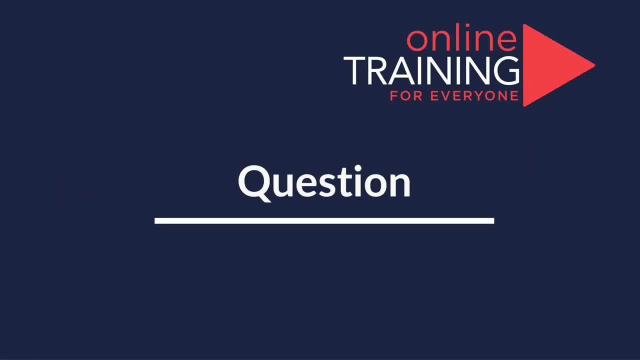 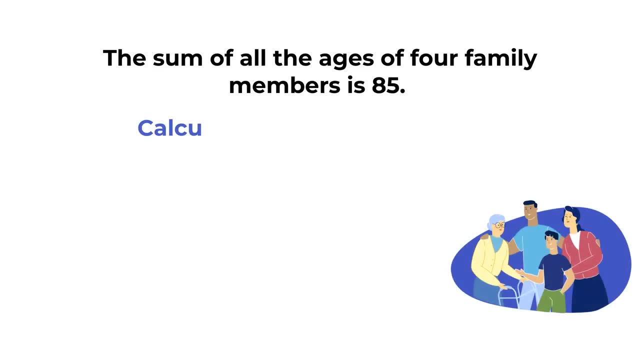 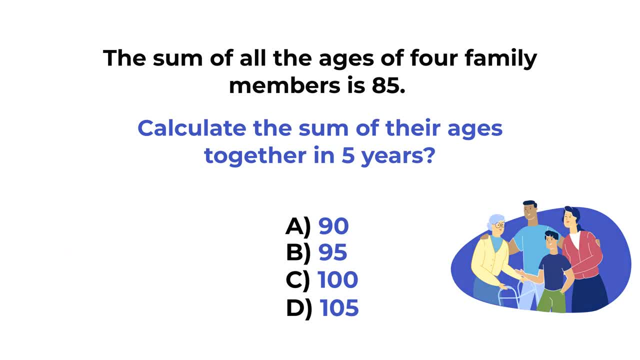 Here's the puzzling question. If you can calculate the answer to this question, please make sure to post it in the comment section of this video. Thanks for participating and good luck. Ready or not, I'm moving forward to get to the correct solution together. 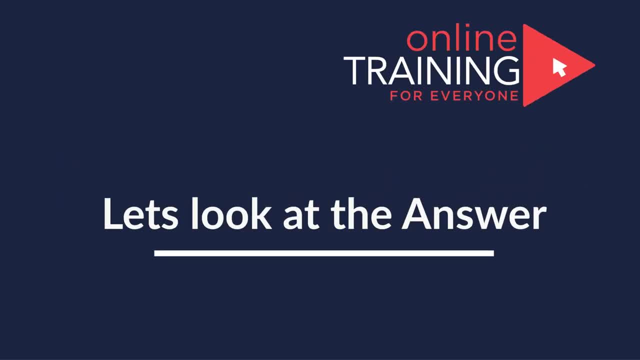 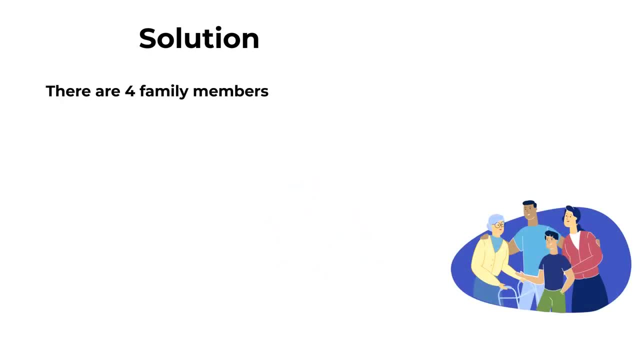 What's interesting about this problem is that it is simpler than you think. So the key here is not to overthink the problem. There are four family members and the sum of their ages is 85. And in five years, each family member will be five years older. So incremental age increase for all family members can be calculated as 4 for family members multiplied by 5.. So incremental age increase for all family members can be calculated as 4 for family members multiplied by 5. by five, five years equals 20 years. 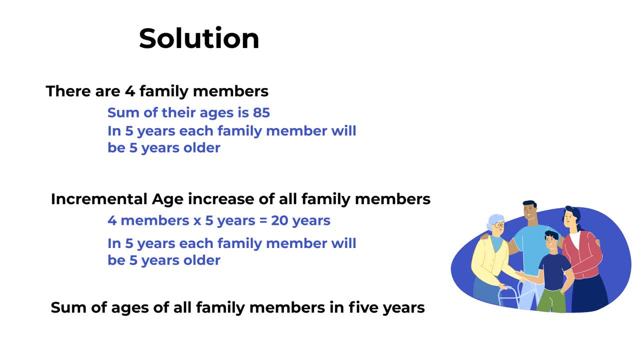 So sum of the ages of all family members in five years can be calculated as 85,, which is original sum plus 20, which is the incremental age increase, and would be equal to 105.. So the correct choice here is choice D, 105.. 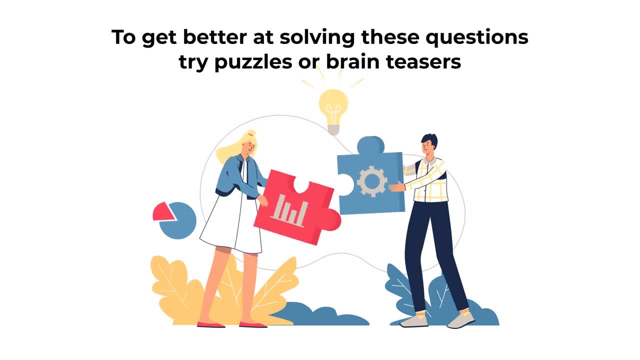 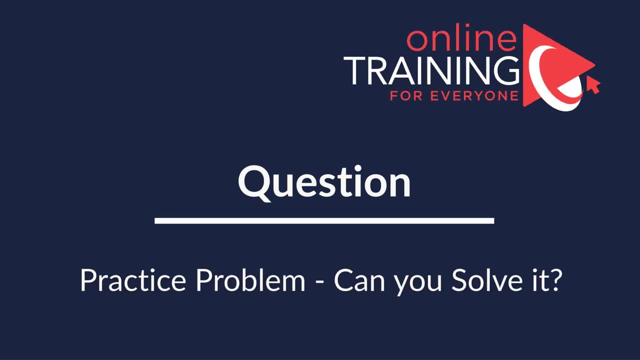 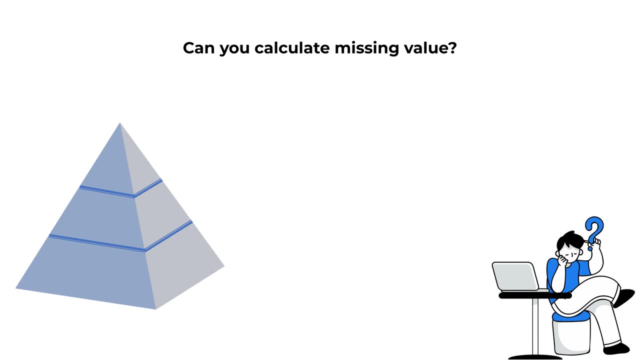 Hopefully you've nailed this question and now know how to answer similar puzzles on the test. And now here's the question for you to practice. You're presented with triangle which is broken down into three equal horizontal parts On the left side of the triangle. 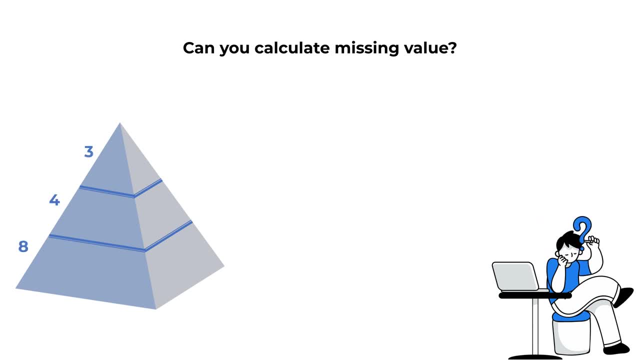 you see numbers eight, four and three. if you go from the bottom to the top And on the right side of the triangles, you see numbers two, six and one number is missing. You need to select missing number from four different choices. 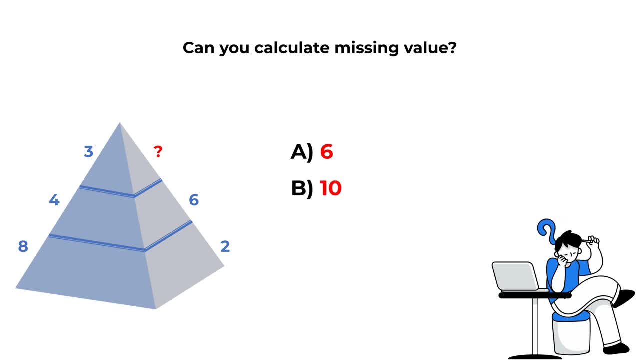 Choice A: six, Choice B: 10. Choice C: seven And choice D: two. Give yourself a little bit of time to see if you can come up with the solution. If you figured out the solution, please make sure to post your answer. 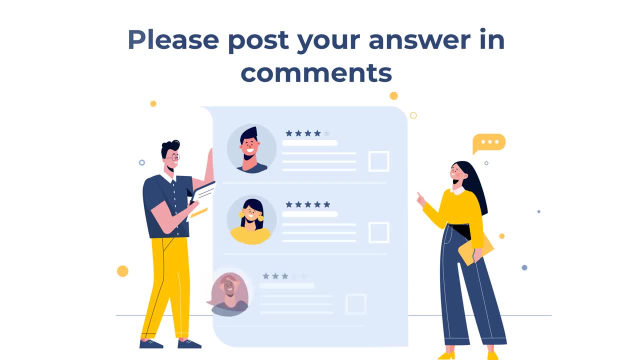 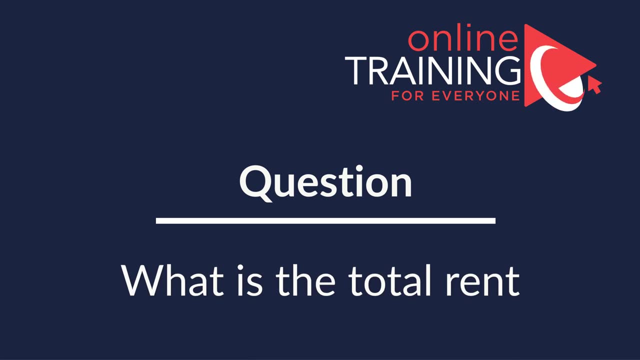 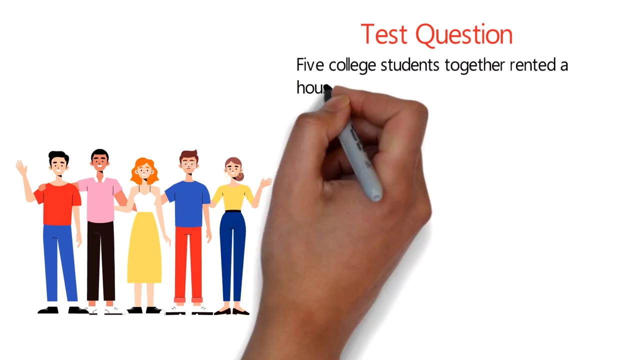 in the comment section of this video so I can give you my feedback. Thanks for participating and good luck. Here's an interesting question You may need to know, not just for the test, but also if you're trying to rent the house. Five college students together rented a house. 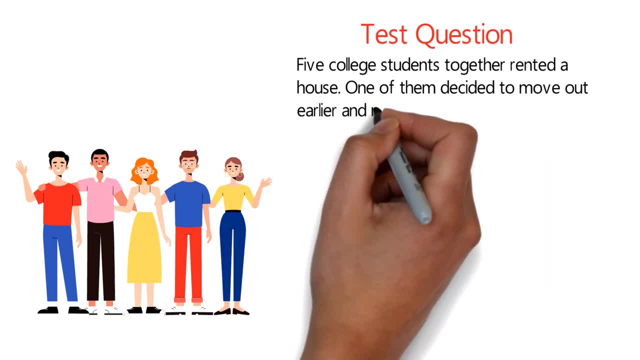 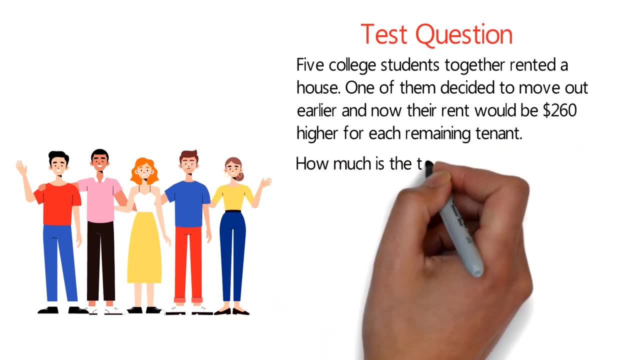 One of them decided to move out earlier, and now the rent would be $260 higher for each remaining tenant. What is the cost of the total rent, considering the rent is shared equally among students And you're presented with four different choices. Choice A: $5,200. 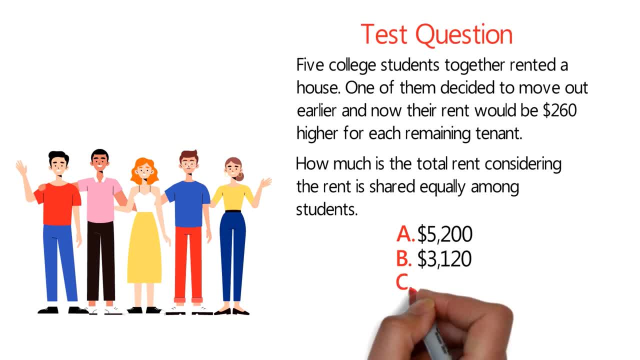 Choice B: $3,120.. Choice C: $2,600. And choice D: $2,950.. two thousand three hundred and forty dollars. give yourself 20 to 30 seconds. maybe pause this video to see if you can come up with the answer on your own. let's go ahead and solve this challenge. 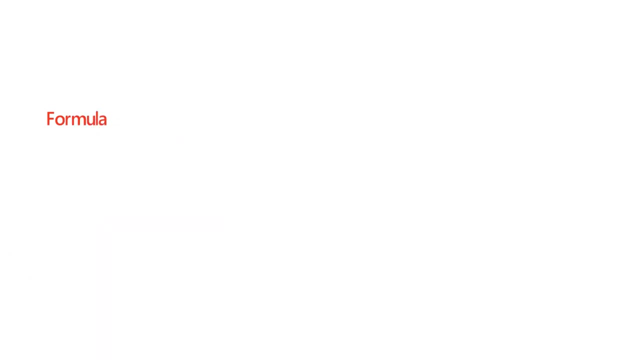 together. one of the easiest way to solve this challenge is to create a formula. let's start by defining a variable, and we will define this variable as s, which would represent an initial split trend for five students. so, using this formula, we can calculate the total house rent. 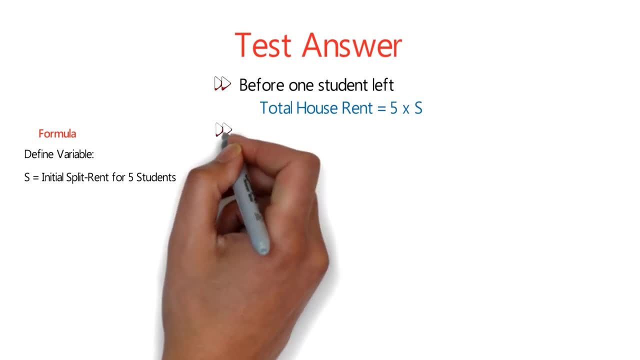 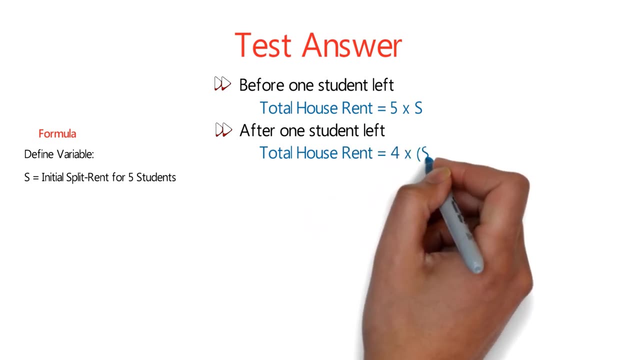 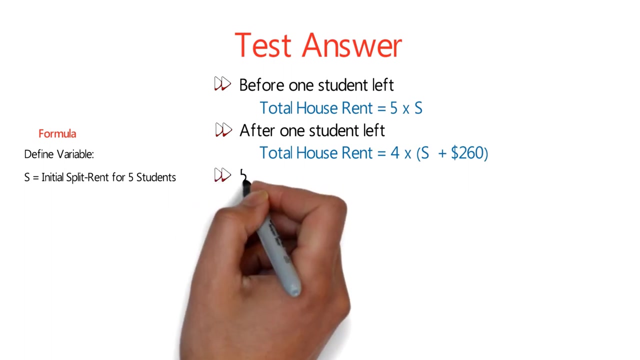 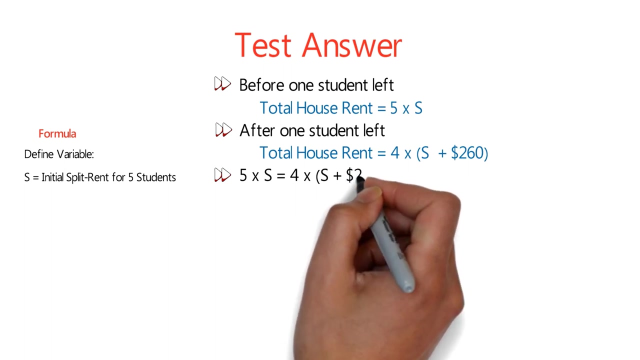 as five multiplied by s, which means that after one student left, the total house rent could also be calculated as four multiplied and then the value in parentheses s plus 260. using both approaches we can create an expression: five multiplied by s equals four multiplied and then the value in parentheses s plus 260. once we simplify it, we'll get to the equation. 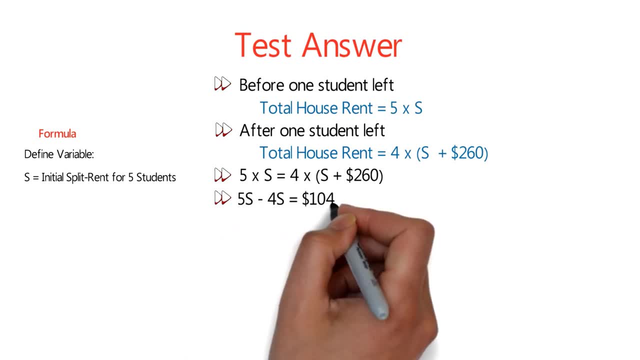 5s minus 4s equals 1040 dollars, which means that the s equals 1040 dollars, which represents initial one student trend. to calculate total house rent, we need to multiply five by one thousand forty dollars and the result will be five thousand two hundred dollars. 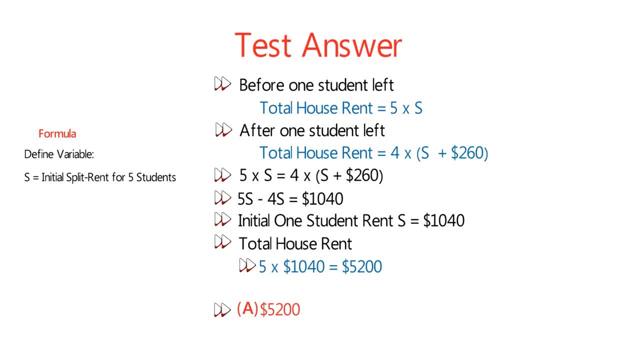 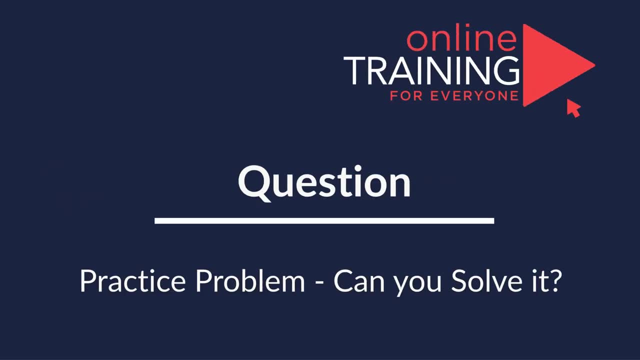 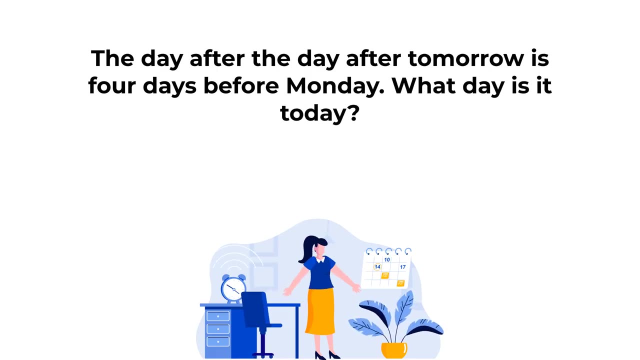 so the answer is choice a: five thousand two hundred dollars. hopefully you've nailed this question and now know how to answer similar. here's the practice problem for you: the day after the day after tomorrow is four days before monday. what day is it today? you have four different choices. 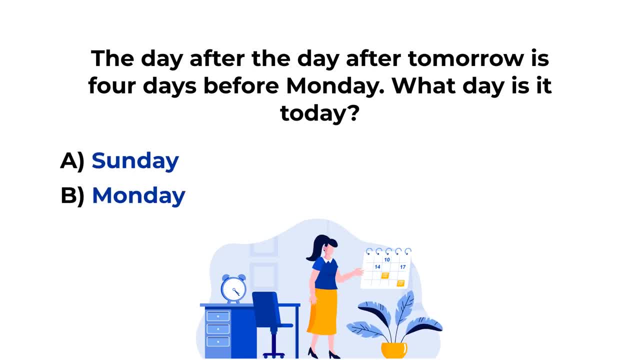 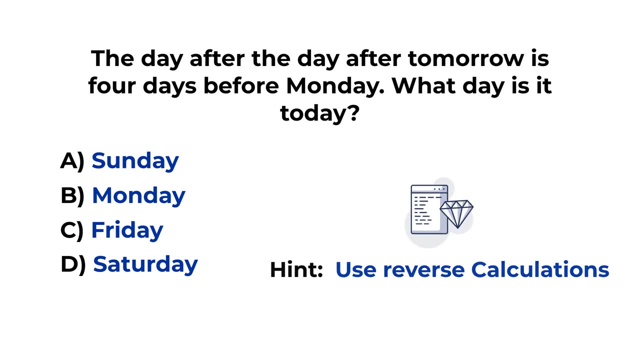 choice a- sunday. choice b- monday. choice c- friday. choice d- saturday. feel free to pause this video to see if you can come up with the solution. i would like to give you a hint. the best way to solve these types of problems is using reverse calculations. so do you see the answer? give yourself 10 to 15 seconds to. 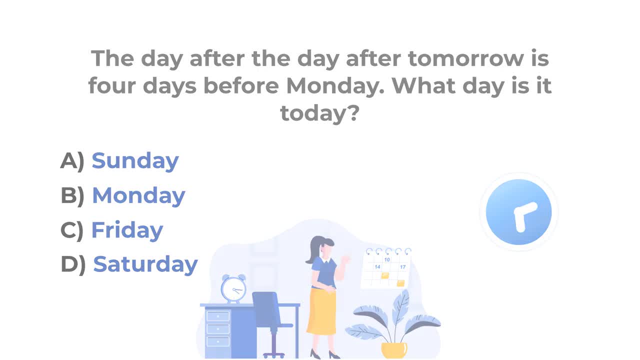 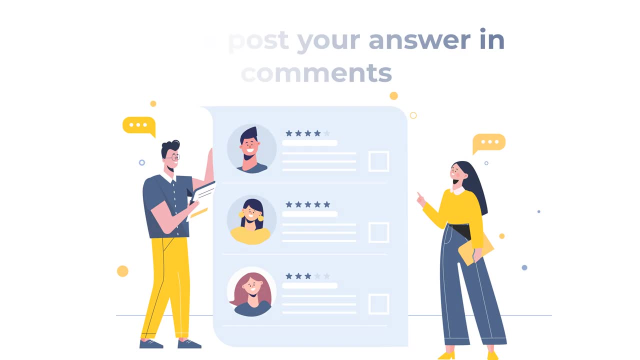 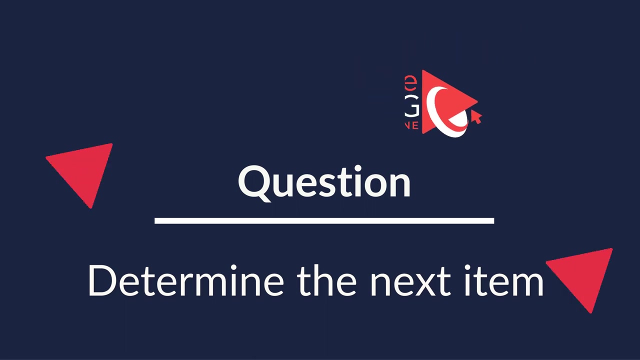 see if you can come up with the solution. did you figure out the answer? make sure to post your answer, as well as your rationale for solving this problem, in the comment section of this video. thanks for participating and good luck. very frequently on the test you might get a question to determine the next item in the series. 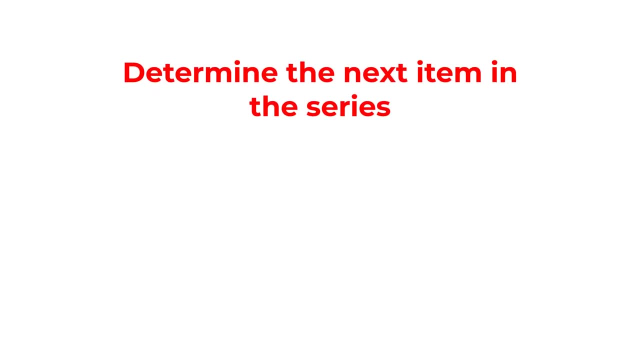 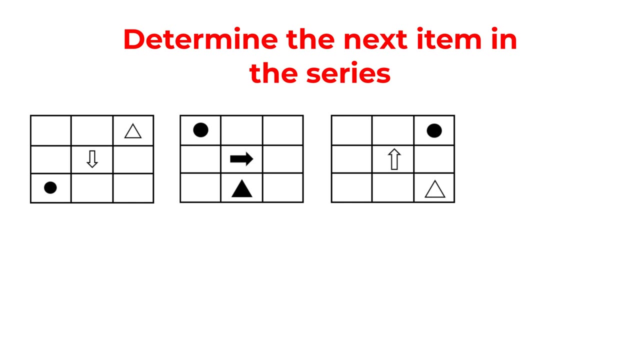 we are looking at exactly this type of question here. you are presented with the series of three by three matrices. each matrix has circle, arrow and triangle inside, and your goal is to determine matrix number four in the series. you're presented with four different choices: choice a, b, c and d. 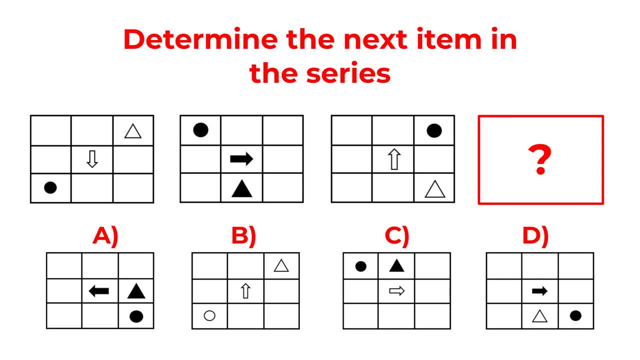 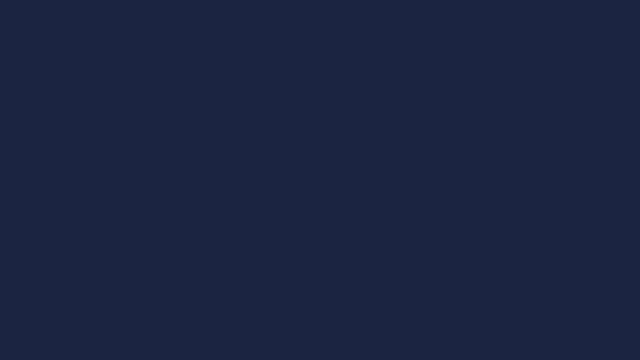 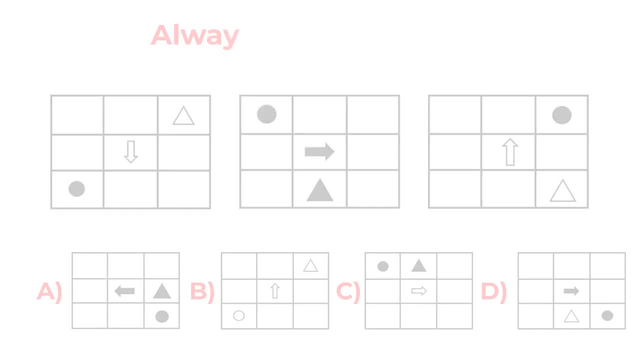 take a close look and see if you can determine the pattern ready or not. i'm going to move forward and share with you the correct answer, at least from my standpoint. when solving these types of challenges, we need to like all behaviors of the picture- anything but colors- in the format we know a good for when solving these types of challenges. my 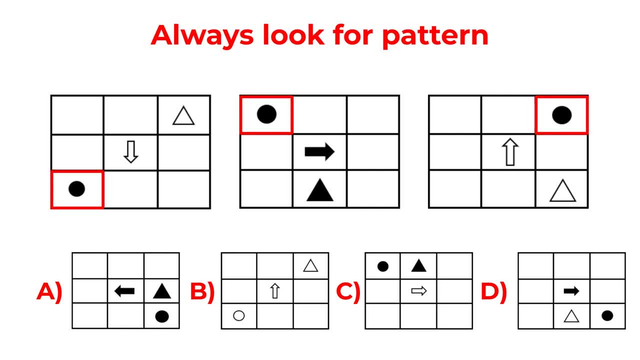 advice to you: always look for patterns, and there are multiple different patterns here for each shape. circle, for example, changes places but always remains black and always filled with color. triangle changes places in the matrix but changes from filled with black color to non-filled with black border. an arrow rotates怎麼. 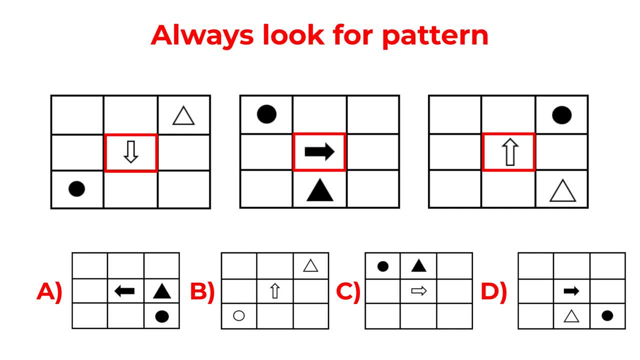 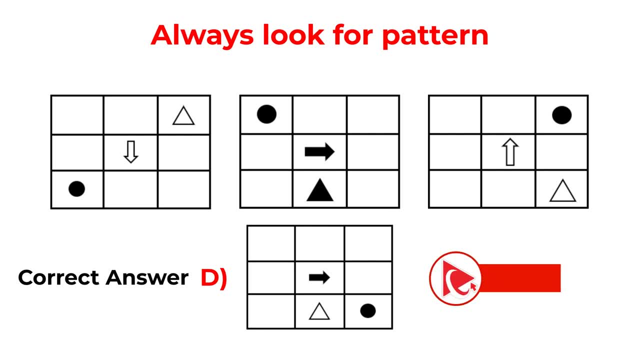 but changes from filled with black color to non-filled with black border. So the correct choice here is choice D. Hopefully you've nailed this question and now know how to answer similar problems on the test, In case you see any other solutions. 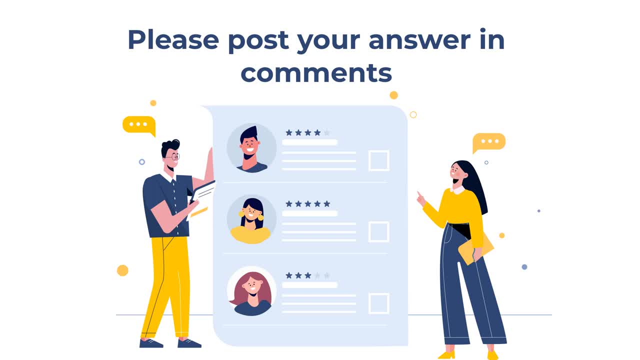 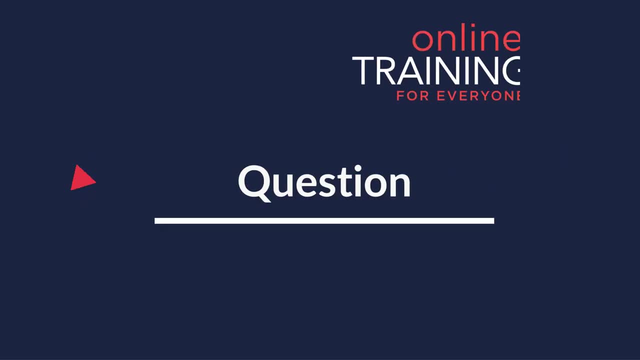 please make sure to post in comments And if you're getting ready for the test, please make sure to check out my e-book. in the description section of this video, Here's an interesting question you might easily get on the test. John's monthly spending is $1,500. 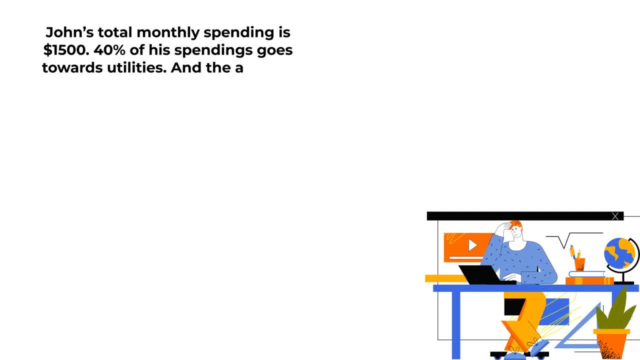 40% of his spending goes toward utilities, and the amount that he spends on heating and electricity is 15% more than what he spends on utilities. How much does John spend on things besides heating, electricity and utilities? You're presented with four different choices. 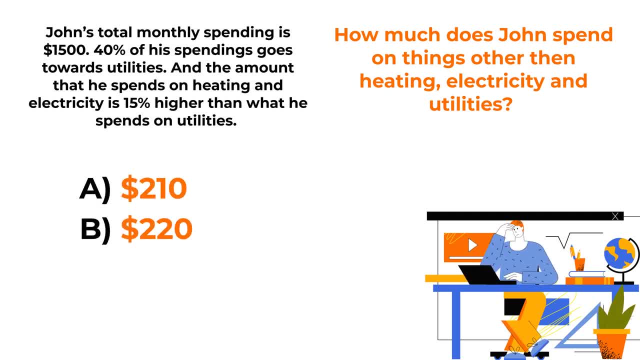 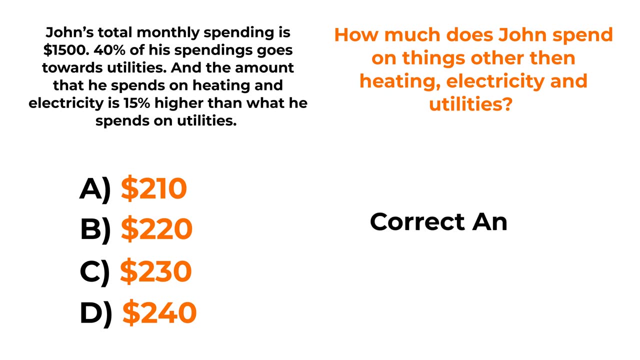 Choice A: $210.. Choice B: $220.. Choice C: $230.. And choice D: $240.. Do you see the answer? Give yourself a little bit of time to see if you can calculate the solution. The correct answer here is choice A: $210.. 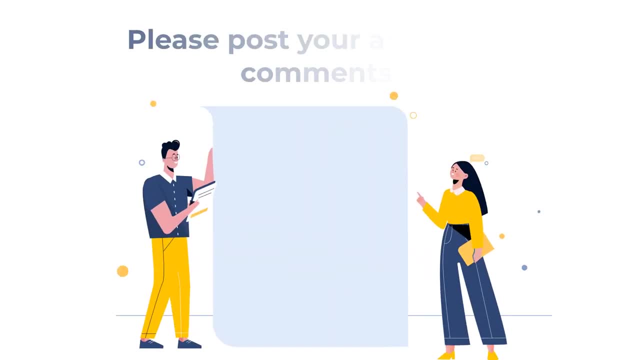 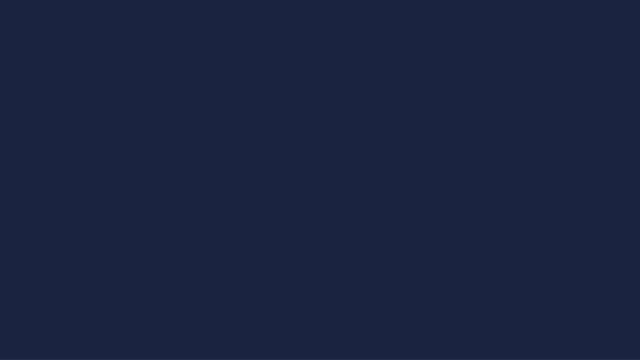 Do you know how to get to this answer? If you figured it out, please make sure to post your answer in the comments section of this video. Thanks for participating and good luck. Here's a very interesting question you frequently see on the test. 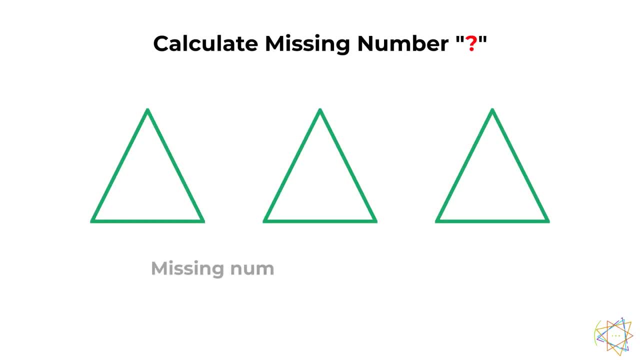 You're presented with three triangles. Each of the corners of each triangle has numbers. For example, first triangle has number 18 on the top, numbers 4 and 2 at the bottom and number 3 in the middle. Second triangle has numbers 56,. 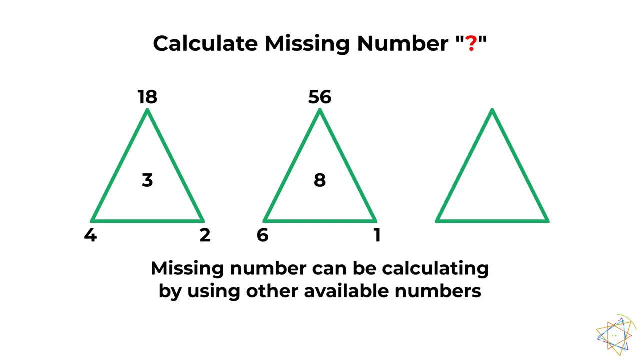 6 and 1, and number 8 in the middle Third triangle has number 104 on the top, number 8 in the middle, number 5 in the bottom left corner and one missing number in the bottom right corner. You need to calculate the missing number. 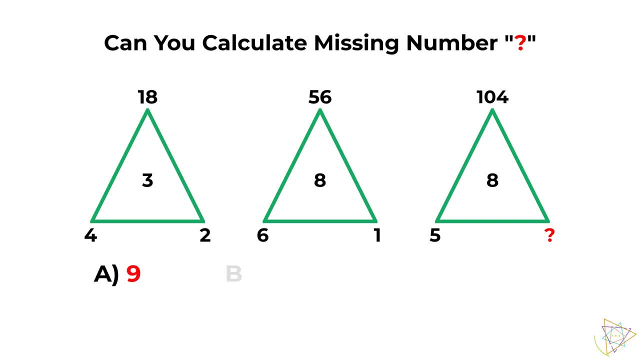 There are four different choices: Choice A: 9., Choice B: 10. Choice C: 11. And choice D: 12.. Do you see the answer? Give yourself a little bit of time to make sure you can come up with the solution. 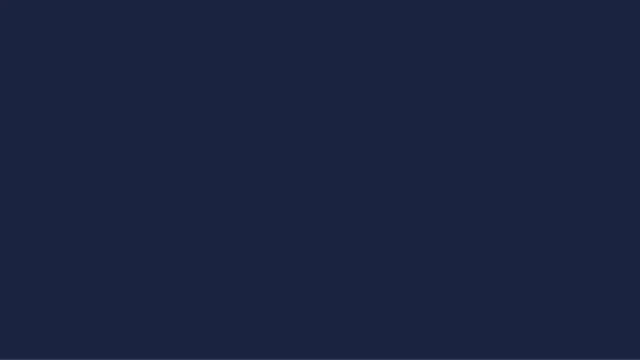 Ready or not, I'm going to move forward so we can solve this problem together. As usual, my advice to you always look for patterns And in this particular problem, the pattern is that the top number divided by the sum of the bottom number, 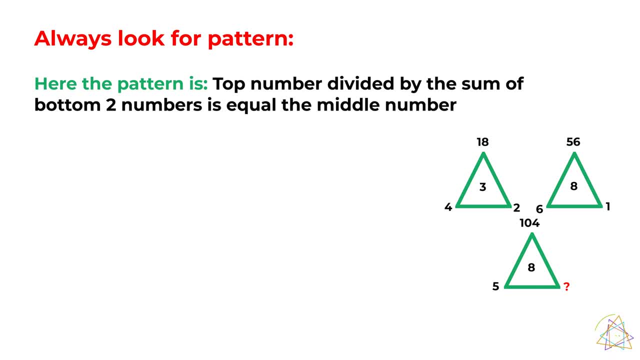 the bottom two numbers is equal, the middle number. Let's look at the example. For example, 18 divided in parentheses, 4 plus 2 would be an equivalent of 18 divided by 6 and would result in 3.. 56 divided by the sum of 6 and 1. 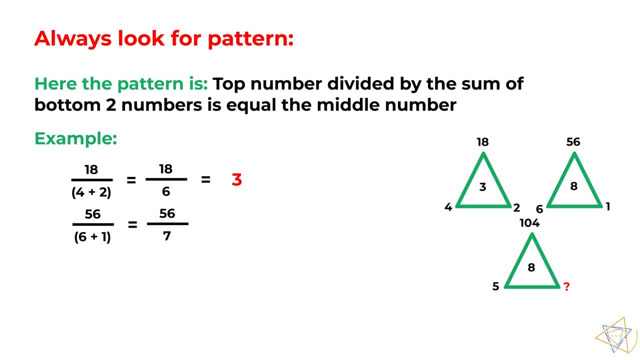 would be an equivalent of 56 divided by 7 and would equal 8.. Which means that we can build a formula And our formula will have 104 on the left divided by the value in parentheses. 3 plus question mark would be equal to 8.. 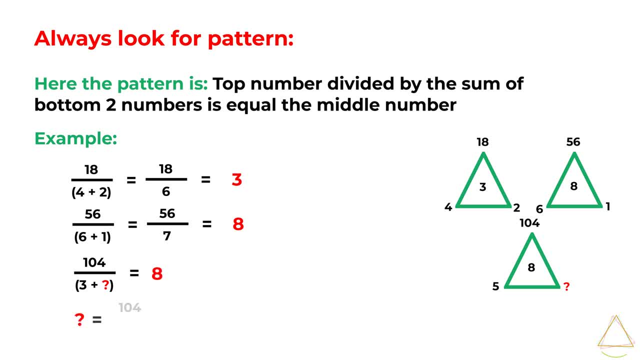 Which means that the question mark would be equal 104 divided by 8 minus 3,, which would be an equivalent of 13 minus 3,, which would be equal to 10.. So the question mark equals to 10. And the correct answer is choice B, 10.. 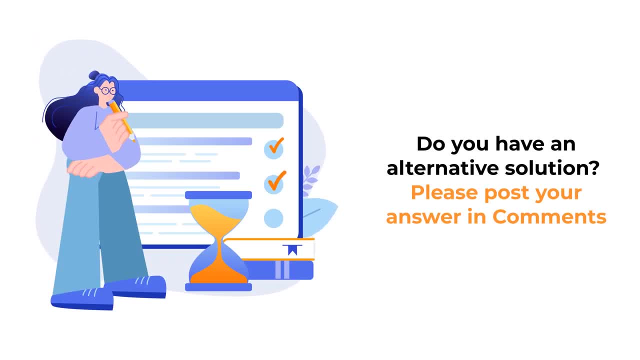 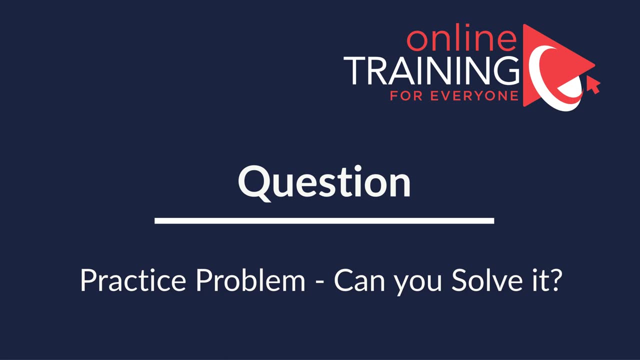 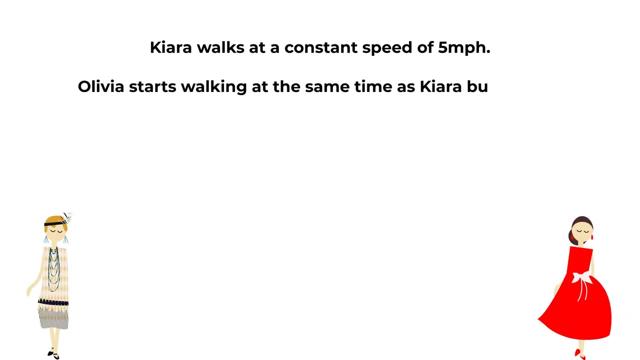 Hopefully you've nailed this question and now know how to answer similar problems on the test. Here's the practice question for you. Kiara walks at the constant speed of 5 miles per hour. Olivia starts walking at the same time as Kiara, but starts 4 miles behind her. 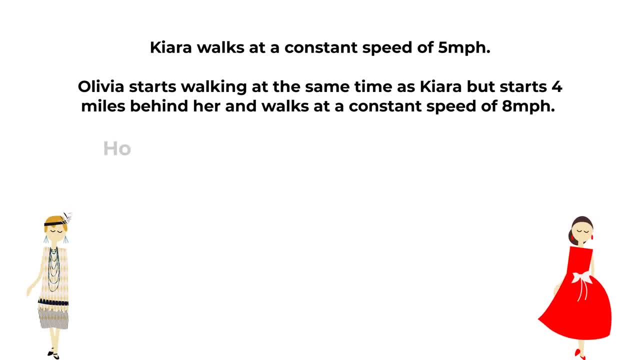 and walks at the constant speed of 8 miles per hour. How long will it take Kiara to catch up with Olivia? And you have four different choices: Choice A- 50 minutes. Choice B- 60 minutes. Choice C- 70 minutes. 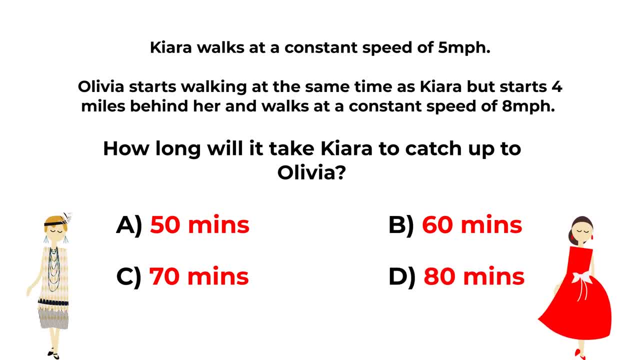 And then choice D: 18 minutes. Please give yourself a little bit of time to see if you can come up with the solution. The answer to this problem is not obvious, But if you came up with the solution, please make sure to post it in the comment section of this video. 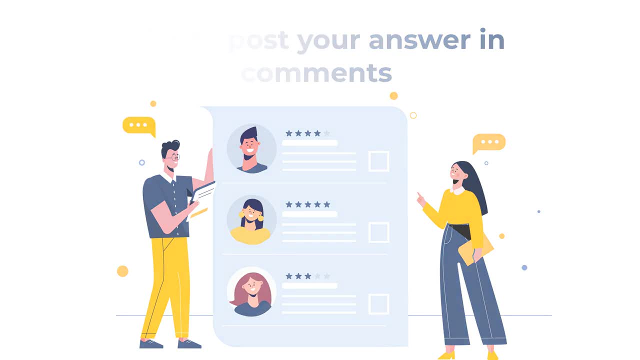 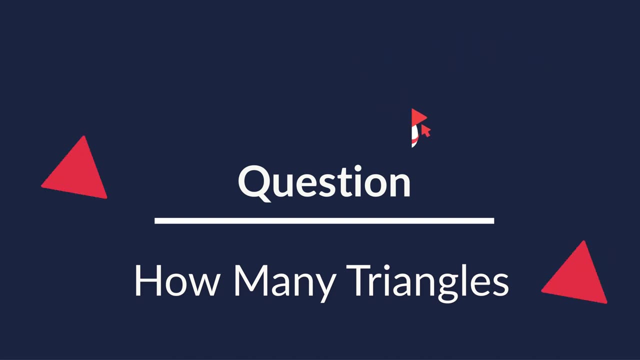 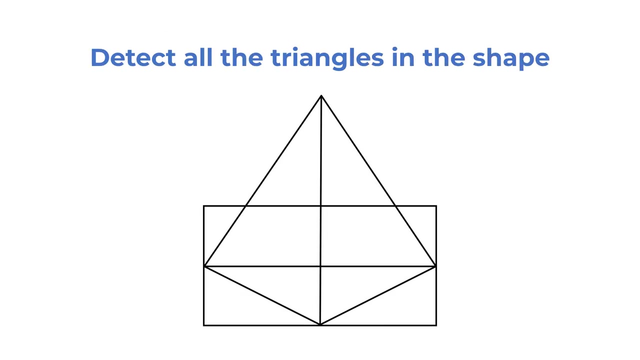 so I can give you my feedback. Thanks for participating and good luck. This particular question was just recently introduced in the test And I would need your help to determine if I answered it correctly. You are presented with the very unusual shape And you need to detect all the triangles. 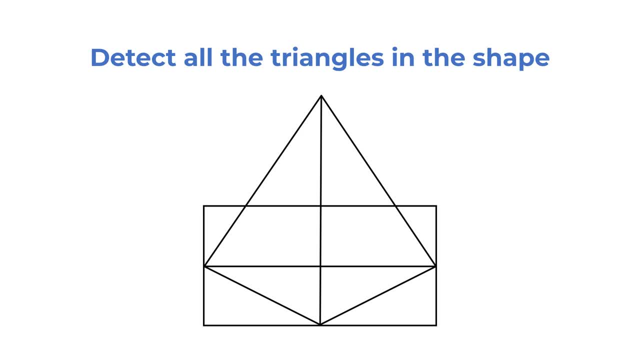 that are part of this shape. You have four possible choices: Choice A: 11., Choice B: 13.. Choice C: 15. And choice D: 17.. Do you see the answer? Consider giving yourself a little bit of time. 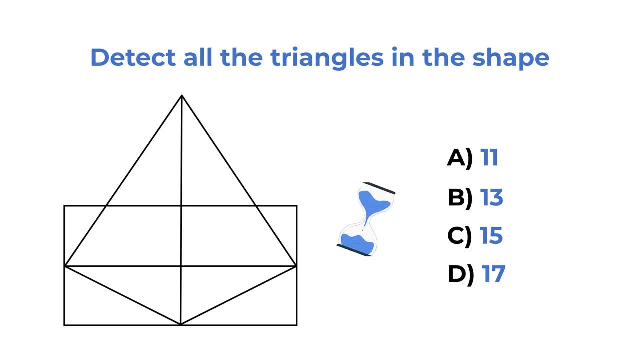 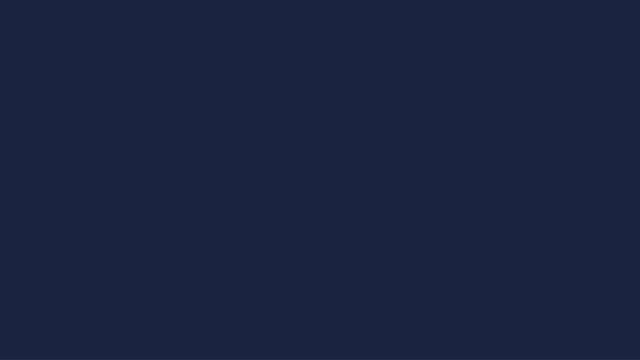 maybe 10 to 20 seconds to see if you can count all the triangles. Ready or not. I am going to move forward and show you how many triangles you will discover. Tricky question, don't you think so? But I was very surprised. 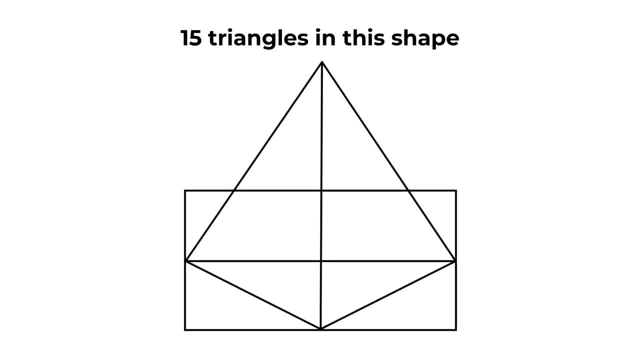 when I counted 15 triangles in this shape. Let me go over and show all of them to you. Here's the first one, Second, Third, Fourth, Fifth, Sixth, Seventh, Eighth, Ninth, Tenth, Eleventh, Twelfth. 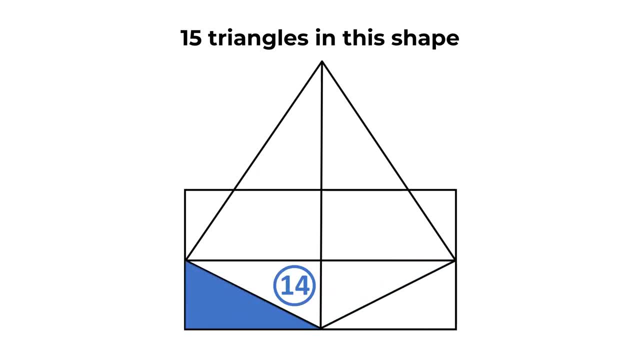 Thirteenth, Fourteenth And fifteenth. Do you see any additional ones? Please make sure to pause them in the comment section of this video And if you are getting ready for the assessment test, please make sure to check out the description. 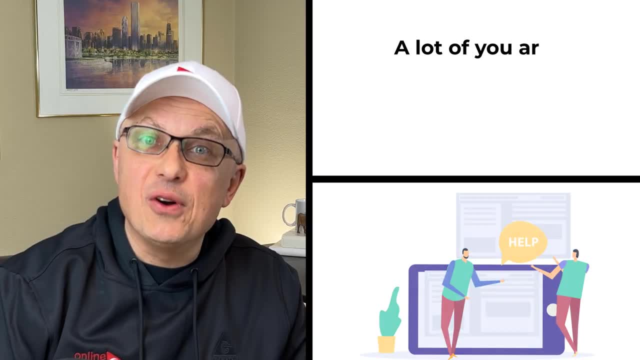 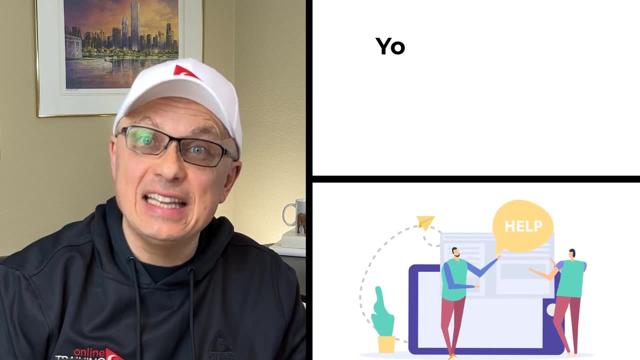 for the link to the e-book that will help you to get ready. A lot of you are interested and ask me: how can I help you? How can I help others? One of the ways you can help other people is by sharing the latest questions. 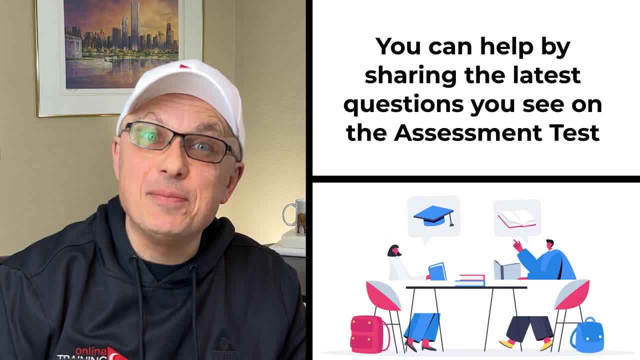 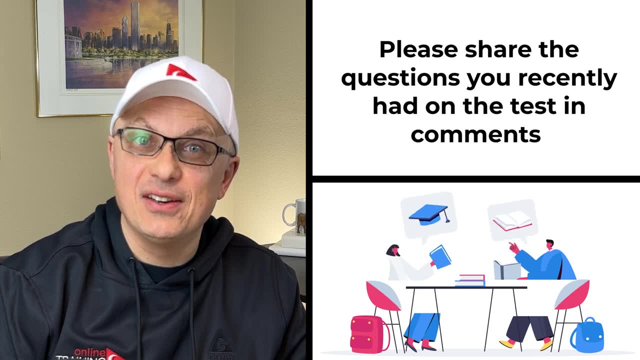 you see as part of the assessment test, And when you share, please make sure to also include how you answered them. Please share the question you recently encountered in the comment section of this video And if you know the answers, please share them as well. 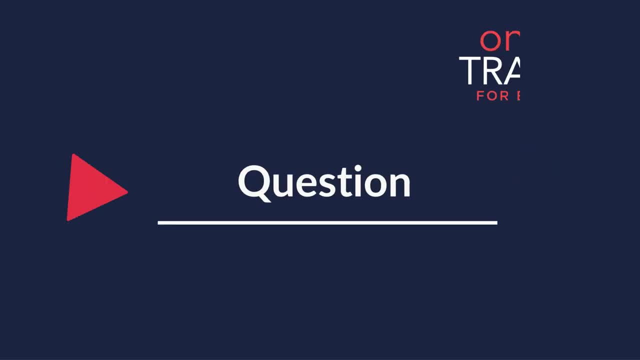 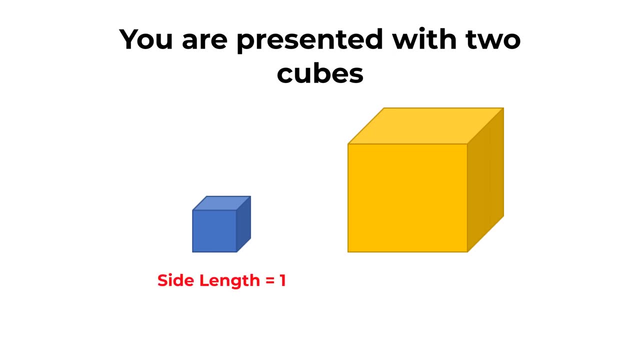 And now let's continue and get you ready for the test. Here's a cool question which you frequently see on the test: One cube has side length equal one unit, And second cube is a larger cube and it has side length equals three units. 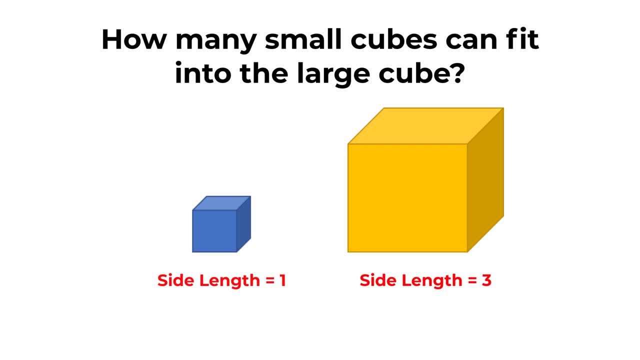 So the question is how many small cubes can fit into the large cube? And you have four different choices: Choice A: 9. Choice B: 18. Choice C: 27. And choice D: 81. Do you know the answer? 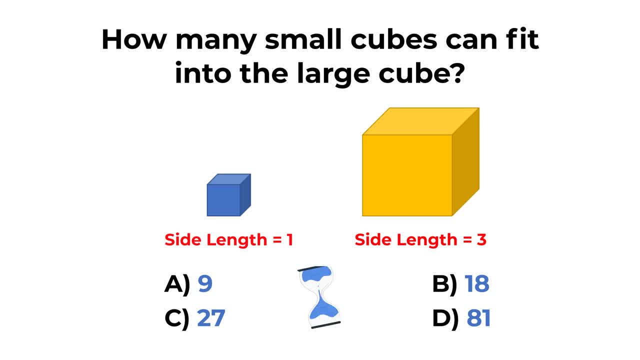 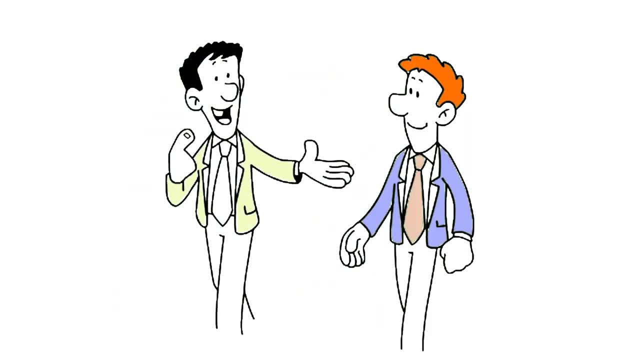 Give yourself few moments to calculate it, Maybe 20 to 30 seconds. This is about as much time as you get in the real test, Ready or not. let's go ahead and get to the correct solution together To solve this challenge. 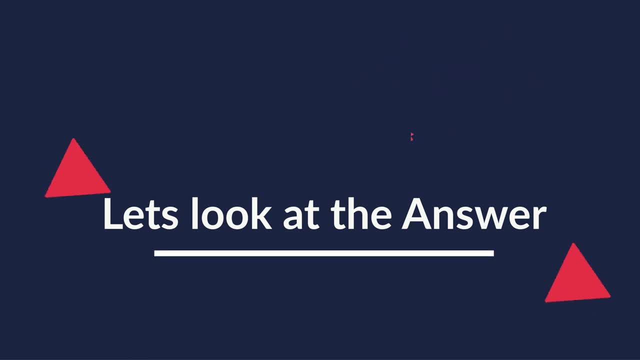 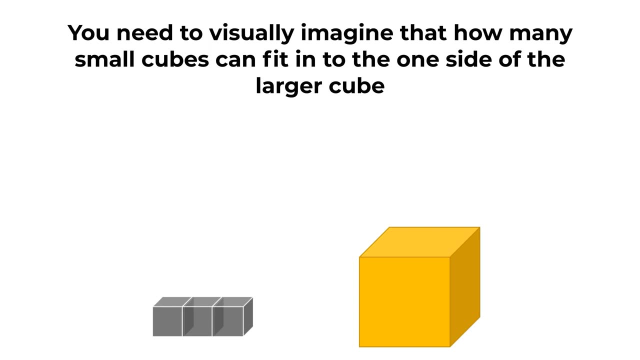 you need to visually imagine how many small cubes can fit into one side of the larger cube And the answer is that three small cubes can fit on each side of the large cube. And since cube is three-dimensional, the number of small cubes that can fit into the large cube 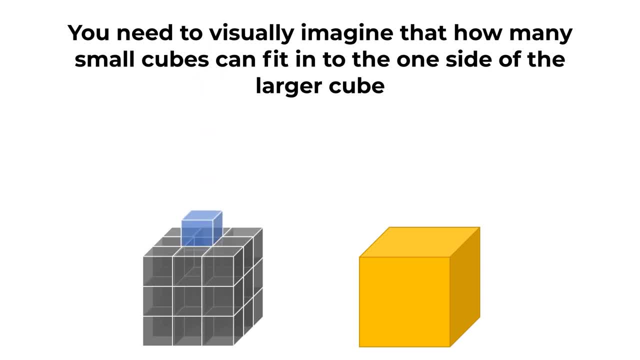 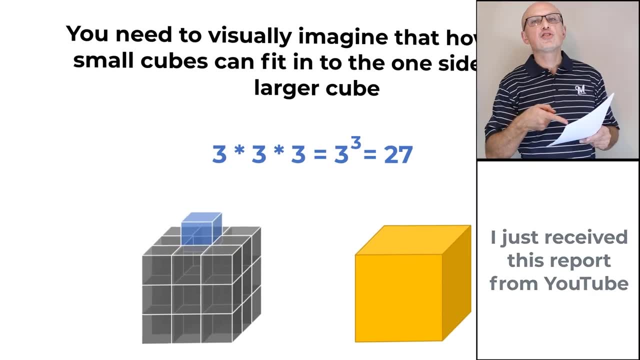 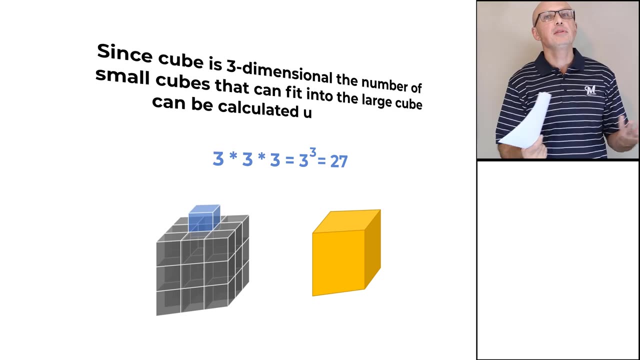 can be calculated using the formula 3 x 3 x 3, which is equal 3 cube- that's where the word cube might be coming from- which equals 27.. Since cube is three-dimensional, the number of small cubes that can fit into the large cube. 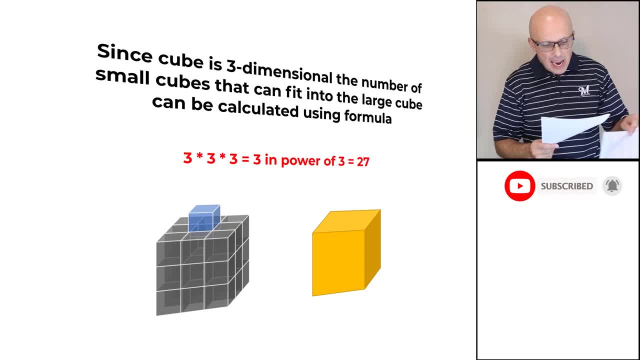 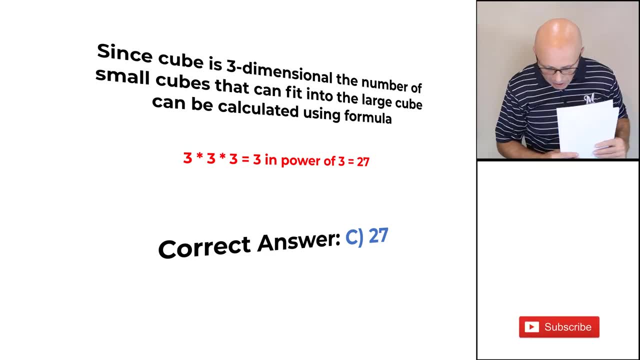 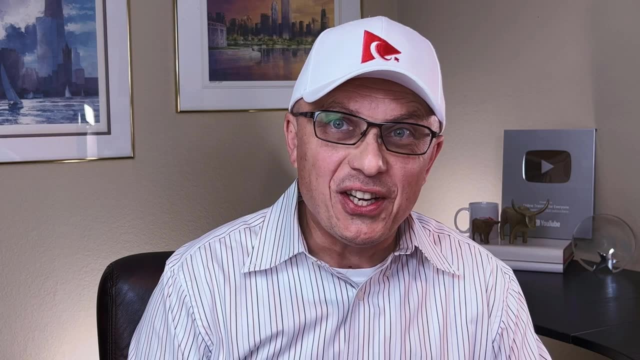 can be calculated using the formula: 3 x 3 x 3 equals 3, cube equals 27.. So the correct choice here is choice C 27.. We nailed this question and now know how to answer similar problems on the test. Thanks for watching. 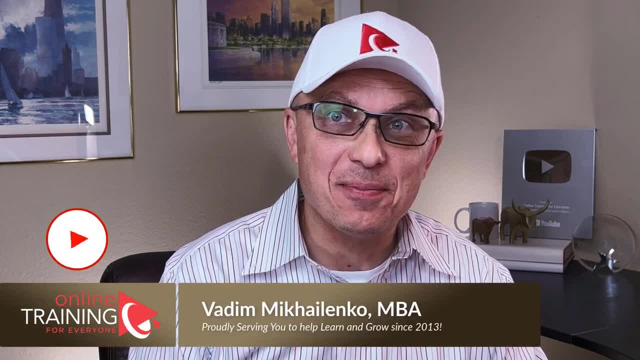 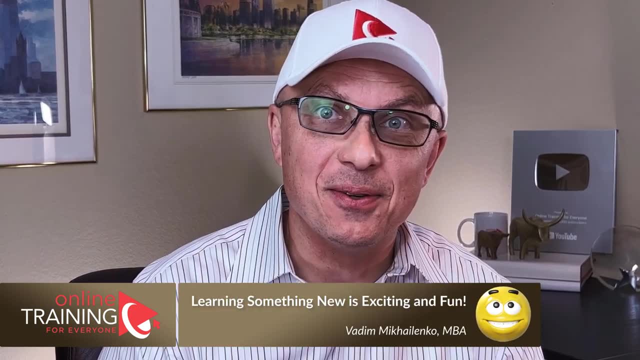 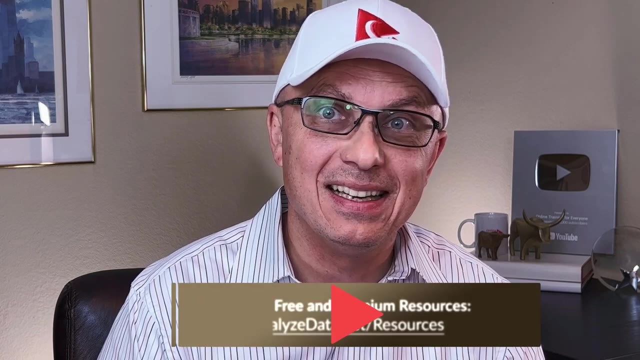 If you like the content, please give us a like and consider subscribing. Thanks for all your endorsement, support and patronage. For additional helpful information, please make sure to check out links in the description For detailed list of available resources. I encourage you to check out.